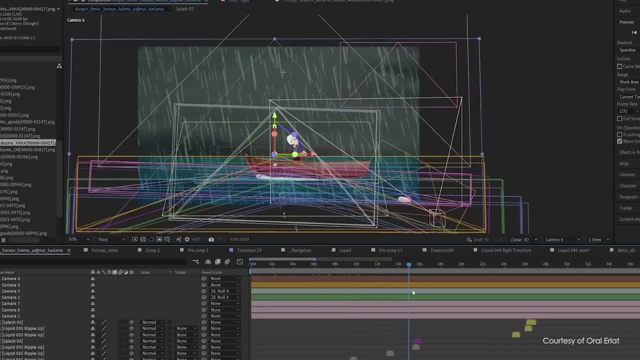 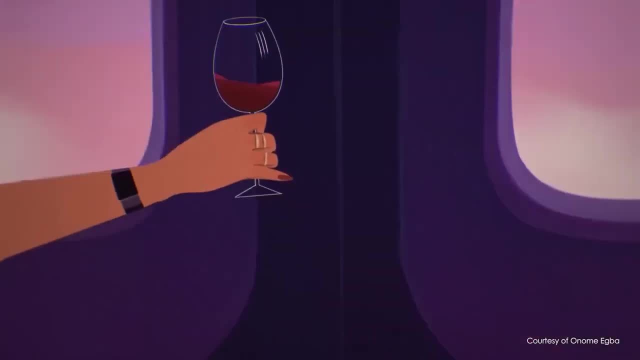 but that doesn't give it justice to how much these software packs enter the hood. It allows you to do so much more. It caters to both beginners and professionals, which means the tools provided are extremely accessible. but if you want to get into the 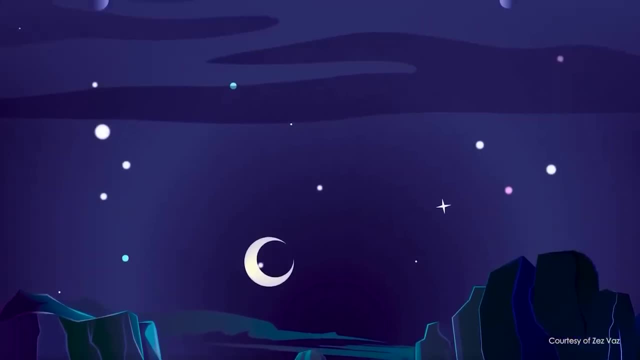 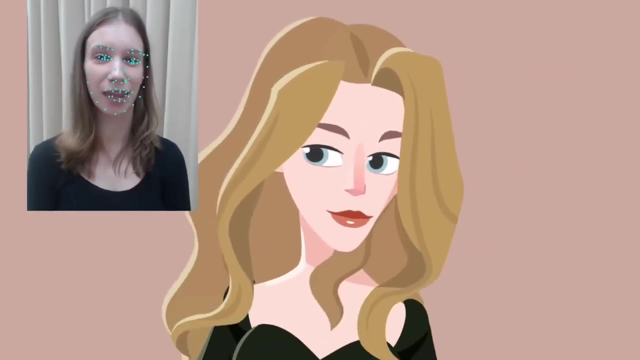 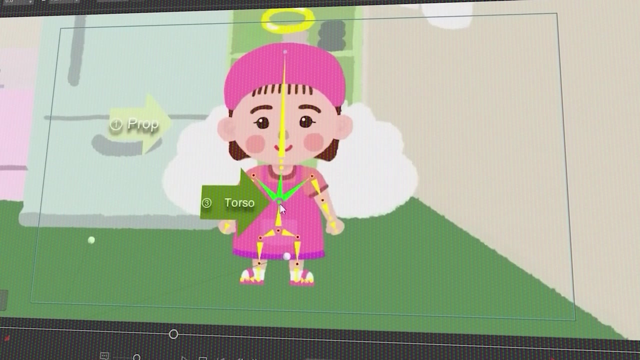 weed and get very technical. Cartoon Animator 5 allows you to do all of that as well. I feel like I find something new every time I launch the software, and that's not to say it is crowded or daunting by any means, One of the reasons that set Cartoon Animator 5 apart from other animation software. 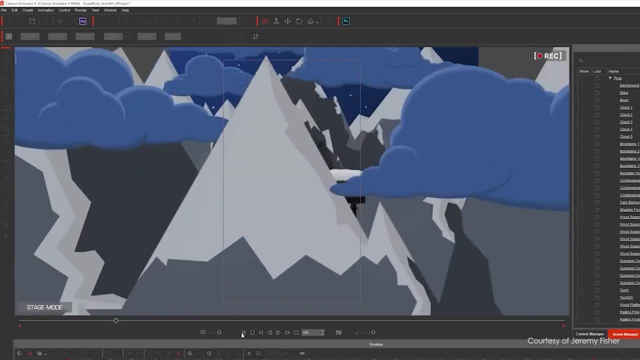 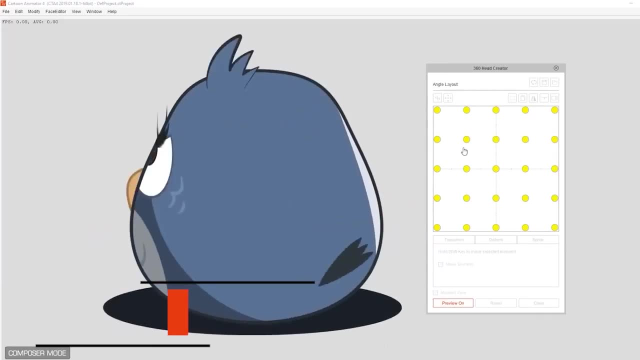 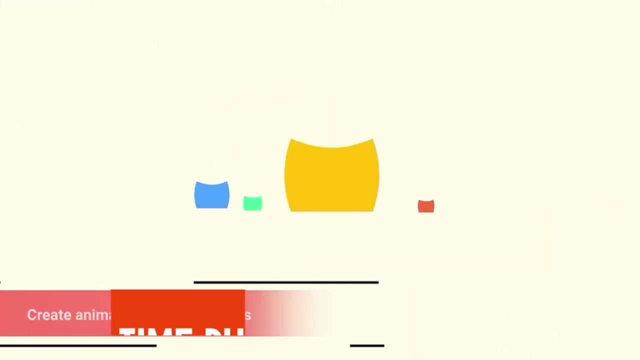 is its ability to always offer new ways for animators to maximize their productivity, whether it is the integration with a 3D workflow, the G3 characters, free-form deformation, real-time physics to add life to your characters, and other things, just to name a few. 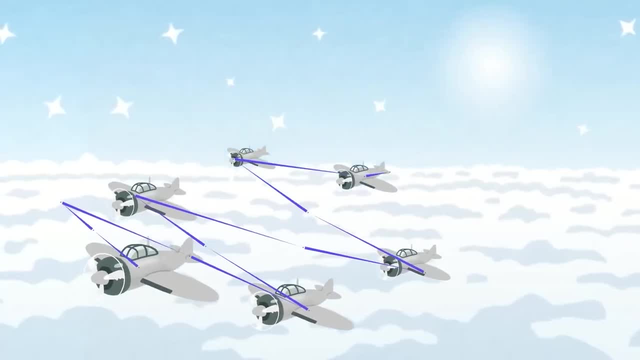 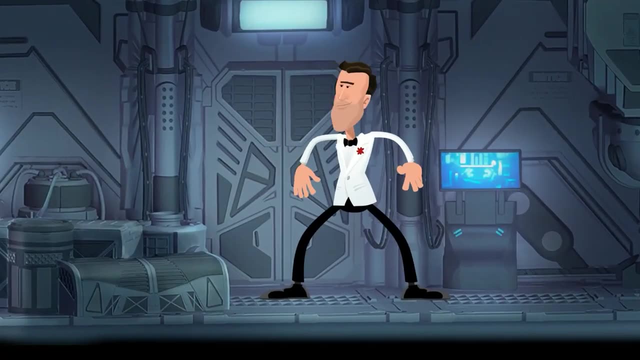 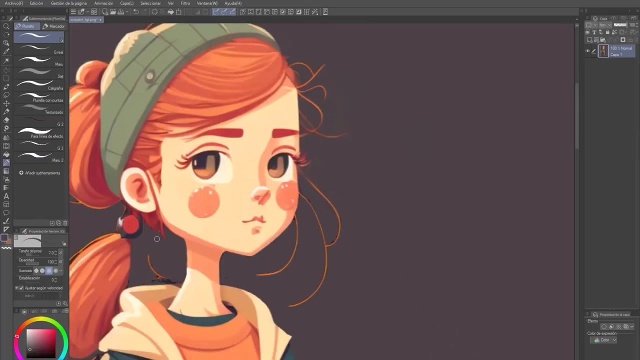 This piece of software never ceases to amaze me with how it can solve so many problems for animators in so many different and unique ways. For example, one of these problems is having to recreate your characters again in Cartoon Animator. but after this update you don't need 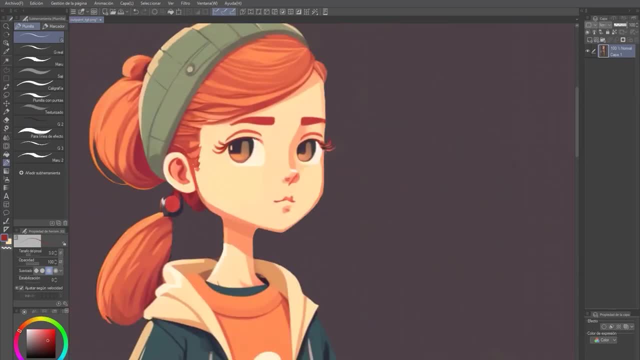 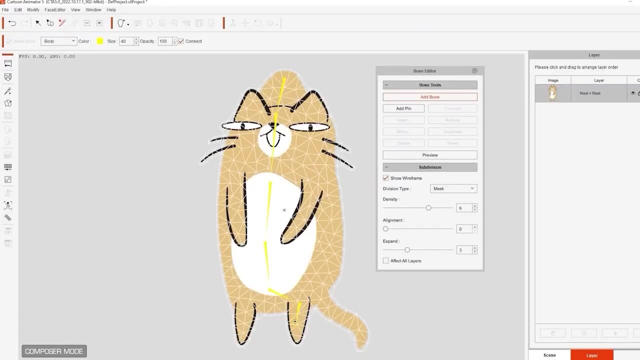 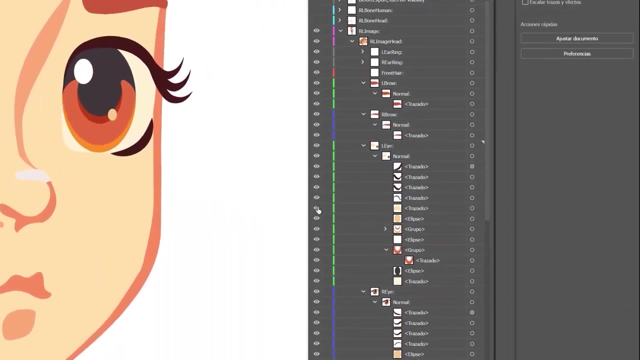 to do so. Cartoon Animator 5 allows you to create animations straight out of the drawing. You can use your favorite SVG-PSD editor to sketch your characters, props and scenes and, in part, import them directly into CTI5. Oftentimes you might think about drawing and animating as two. 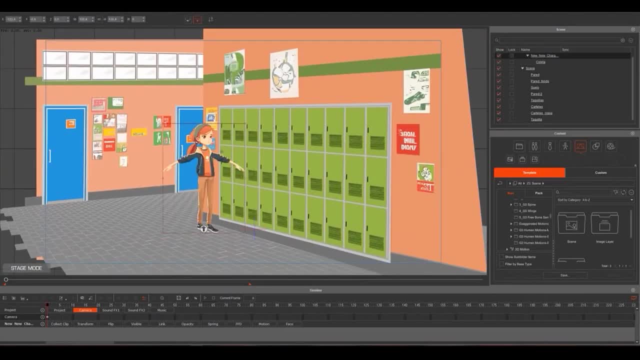 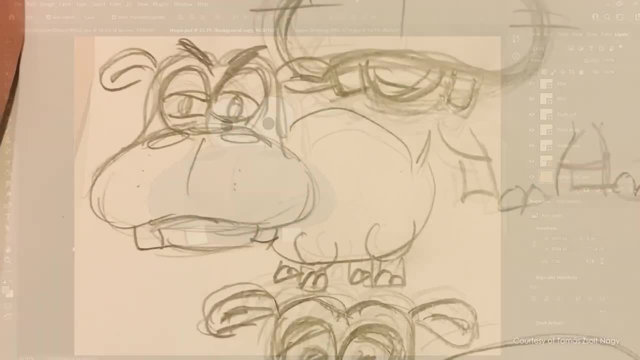 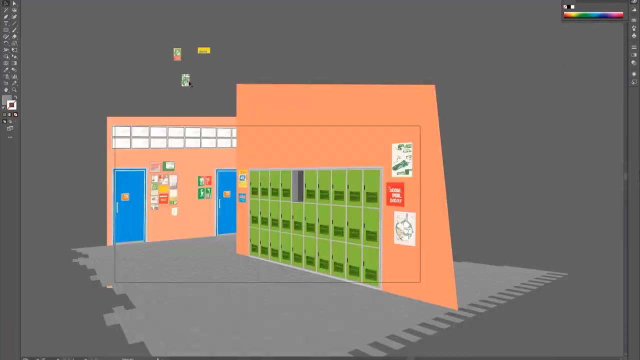 separate things, but you now can think of them as just one thing. Cartoon Animator 5 allows you to create animations straight out of your drawings, Whether it is vector or bitmap. artists can use their favorite SVG or PSD editor to sketch their characters, props and scenes. 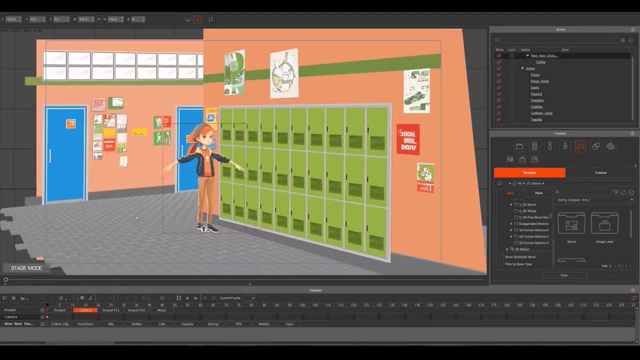 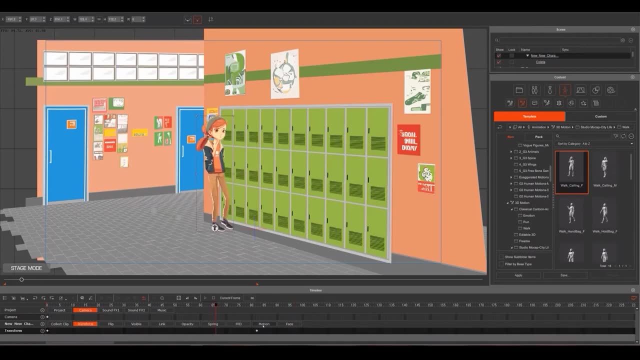 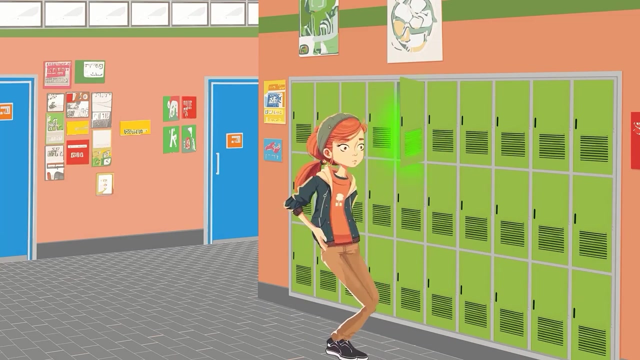 and then import them into Character Animator, which helps you breathe life into your drawings with motion libraries, content that can be dragged and dropped, different assets and much more. Cartoon Animator is bridging the gap between drawing and animation now, because now you can think of them as the same thing, So now you can use your favorite tool. 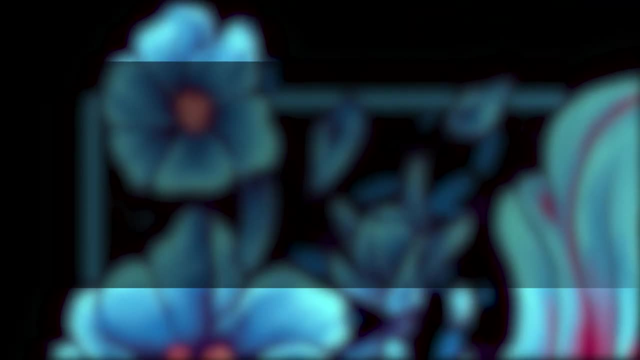 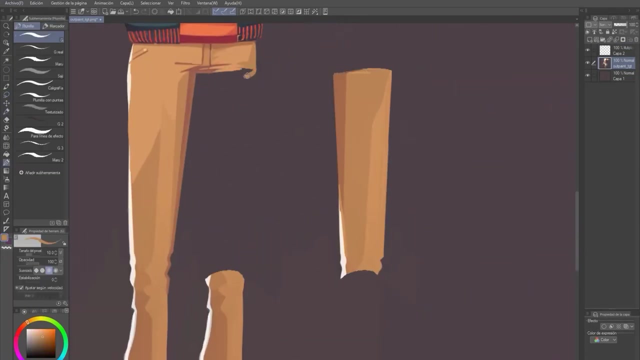 of choice: to draw like Illustrator, CorelDraw, Affinity Designer, Inkscape, etc. And you don't have to worry about where and how. you can create your characters and enjoy the uncompromised details of vector drawing. And if you want to learn more, 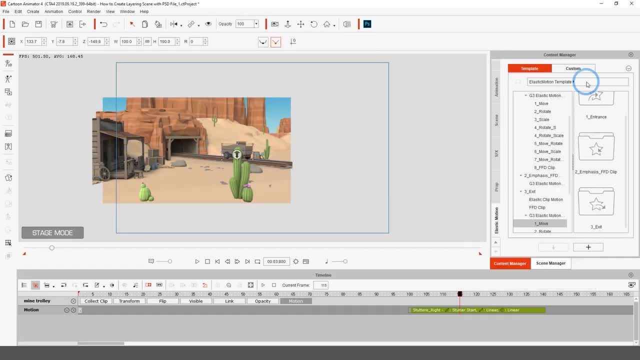 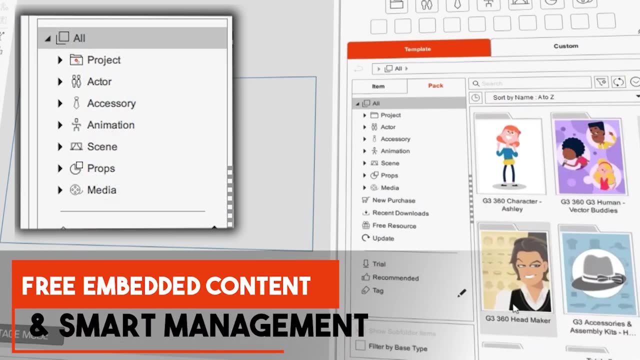 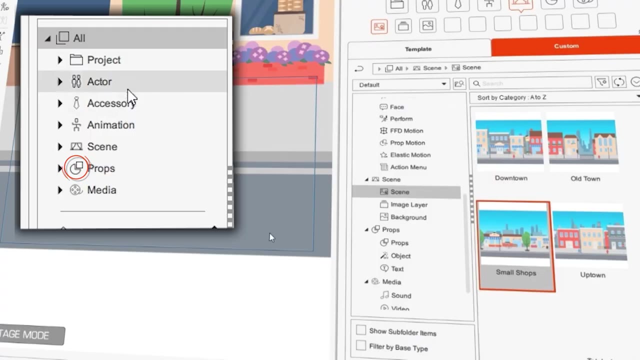 about this. check out this Draw to Animate feature in the link down below Cartoon Animator 5. Cartoon Animator also offers an extensive library of highly valuable demo projects, character assets, accessories, animations, scenes, props and much more- which are ready. 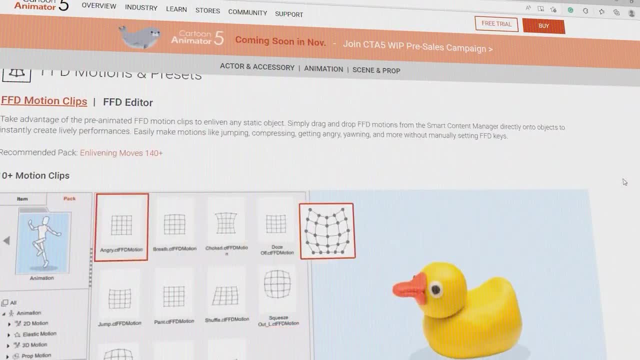 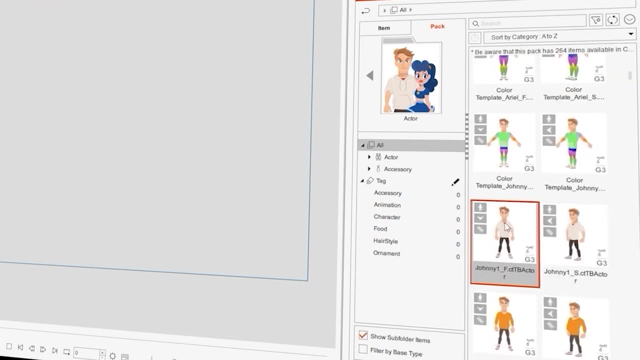 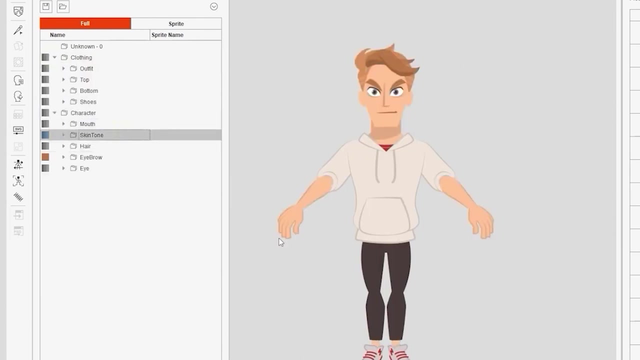 to download from the Smart Content Manager, which contains a ton of free assets. Additionally, there is also a new generation of G3 vector actors, which are coded with the unique color groups and segments, letting you use the color style motif for as many characters as you want. Furthermore, you can easily combine all the assets and elements. 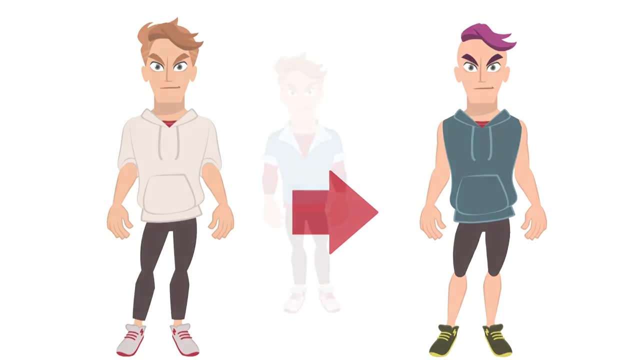 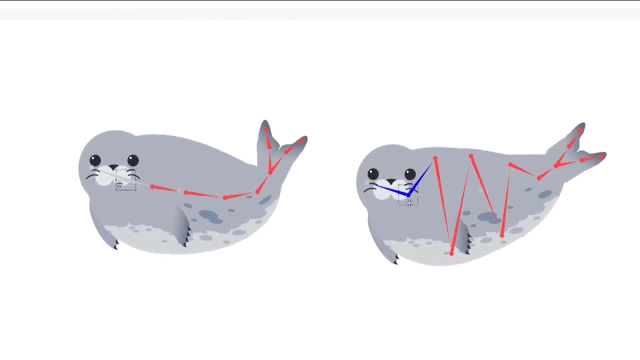 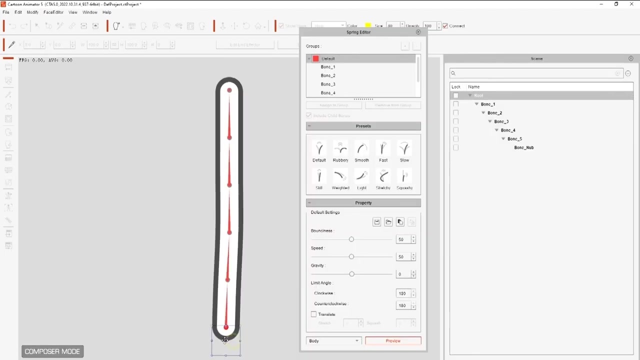 facial components, accessories and props to come up with unique character styles. Cartoon Animator can also save you a lot of time with standard skeletons. A standard skeleton is like a template of bones, but are used to speed up your rigging process for humans, animals, spinal and winged creatures. 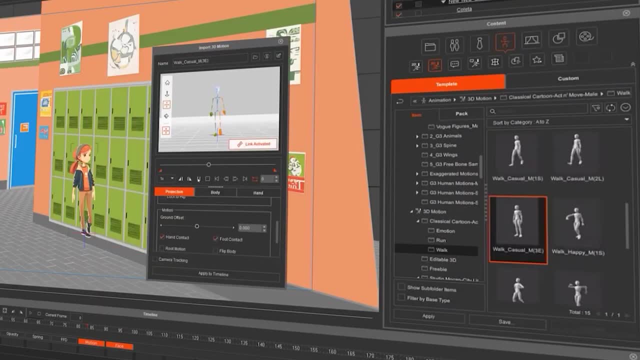 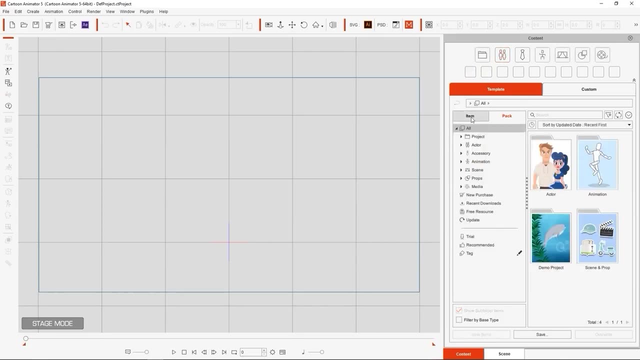 as well as full-face and body templates, which allow you to utilize a huge library of motion across multiple characters. You can think of it as retargeting in Maya or Blender. The shared bone structure just makes a lot of sense. You can find a lot of animations. 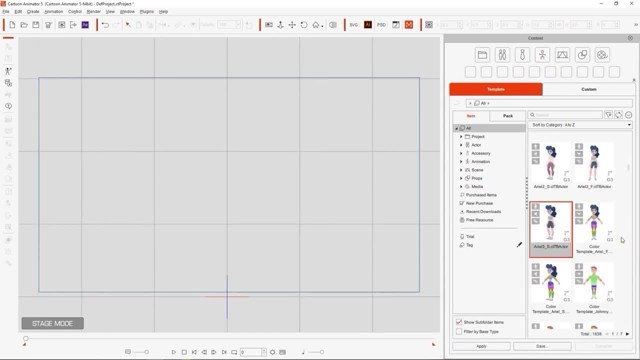 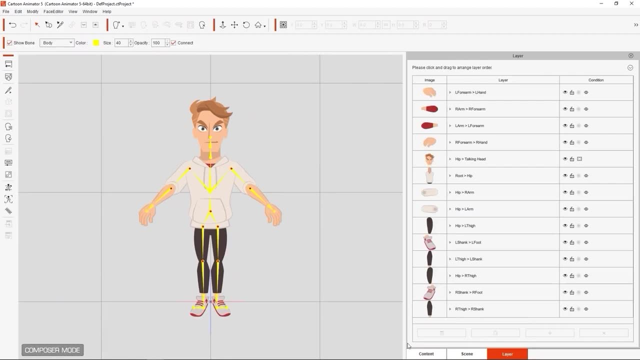 in the Smart Content Manager and you can even browse for more in the Content Store, In addition to the extremely easy auto-character rig importer, where you can rig any 2D character with the free cartoon tool, Or you can take advantage of the many templates that Cartoon Animator is shipped. 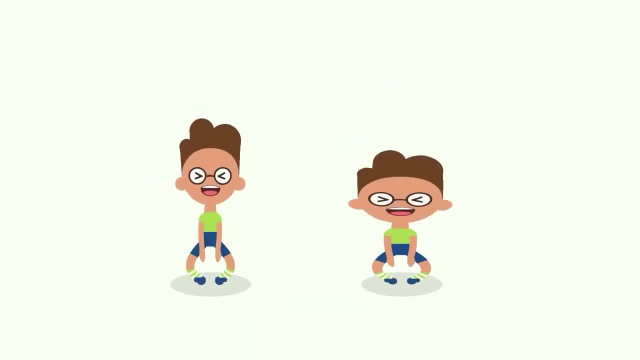 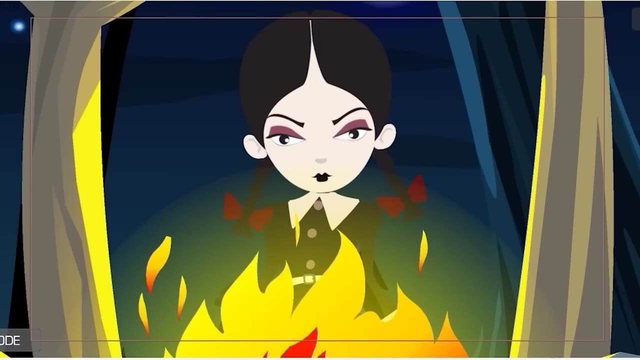 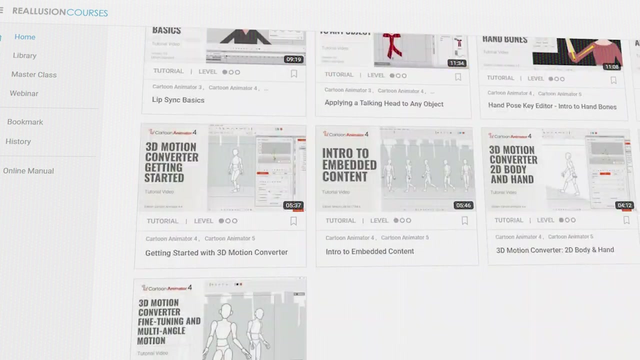 with Cartoon Animator really makes animation more accessible to everyone, because it provides you with the tools necessary to achieve your goal in the least amount of time possible. Furthermore, Reallusion offers extensive courses with a step-by-step guide on how to master each aspect of the software, which is for free, by the way, If you want to check out the Cartoon.